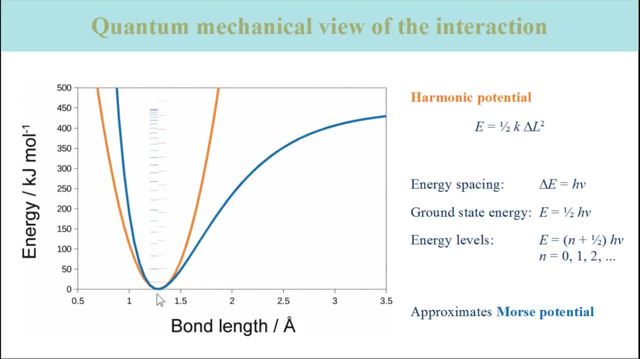 The total energy remains constant and is equal to the maximum potential energy. In the classical world, the total energy can assume any value. However, this is not the case in quantum mechanics, where the energy levels are discrete. The energy levels are shown as orange lines in the figure. 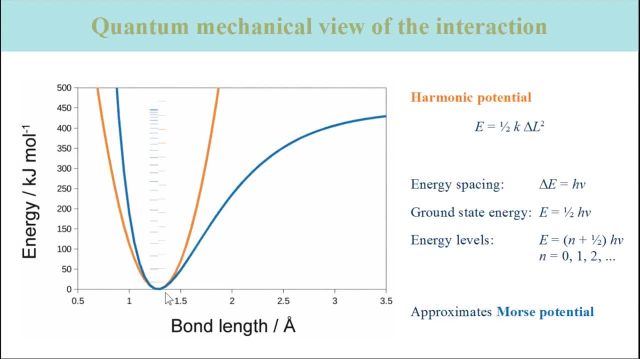 The spacing between the levels is Planck's constant times. the vibrational frequency, The spacing to the next levels is the same, no matter which level we are considering. Another difference from the classical world is the existence of a ground state energy. In classical mechanics the oscillator can be right in the minimum of the potential energy curve. 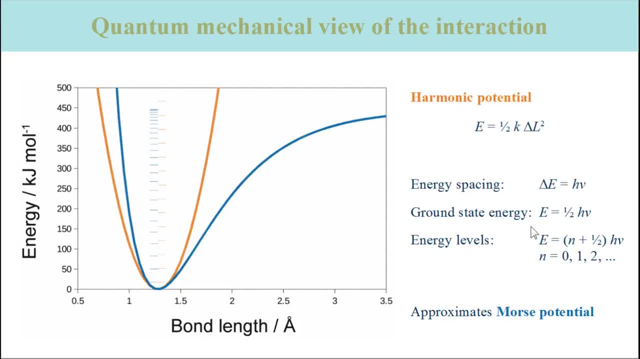 It has no kinetic energy, does not move and the distance is the equilibrium distance In quantum mechanics. the energy of the oscillator can never be lower than half of the energy spacing between the energy levels. Energy spacing and ground state energy together result in the equation for the energy levels of the harmonic oscillator shown here. 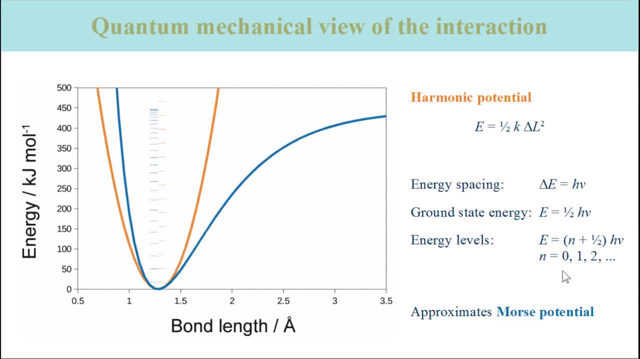 where the counting index n runs from zero over all natural numbers. The harmonic oscillator has no kinetic energy, does not move and the distance is the equilibrium distance. The harmonic potential is an approximation of the Morse potential, which describes the potential energy of a covalent bond much better than the harmonic potential. 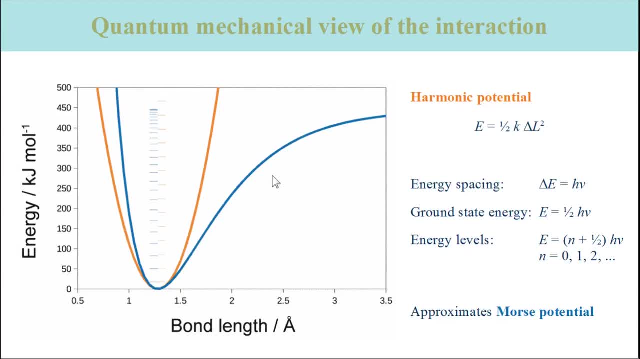 The Morse potential is shown in blue. For short bond distances, the Morse potential is steeper, meaning that the repulsion between the atoms is stronger, whereas it is shallower at longer bond lengths. Importantly, it levels off and becomes constant for large distances between the atoms. 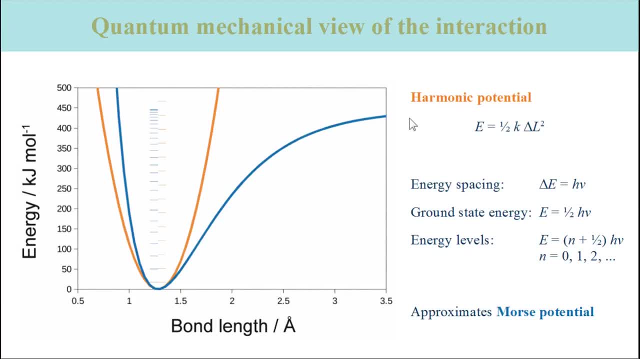 because there is no interaction between the atoms when they are far apart. The Morse potential is an example for an unharmonic potential. This means that the oscillator movement can no longer be described by a simple harmonic movement. Instead, it has to be described by several sinus functions with different frequencies. 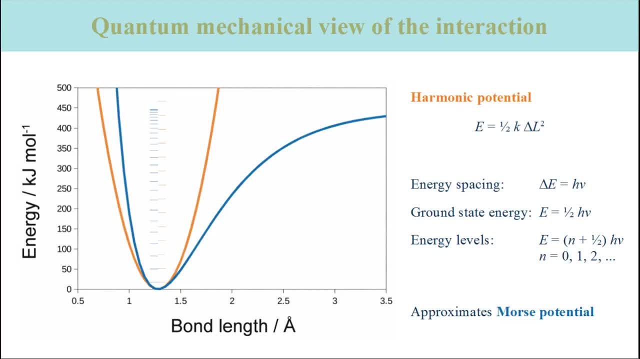 The energy levels of the unharmonic oscillator are also shown in the figure. As you can see, these energy levels in blue are no longer equidistantly spaced. The higher the level, the smaller is the energy difference to the next level. 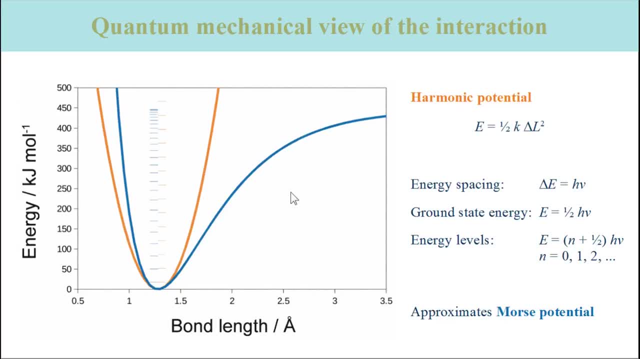 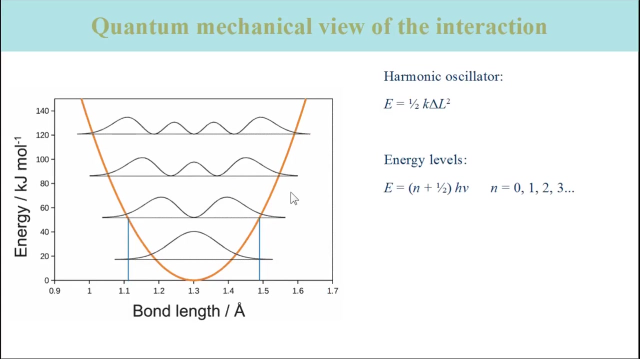 When compared to the energy levels of the harmonic oscillator, those of the unharmonic oscillator are lower. We return now to the harmonic oscillator, because it provides a satisfactory explanation for most features in an infrared spectrum. The figure shows again the potential curve of an aharmonic oscillator. 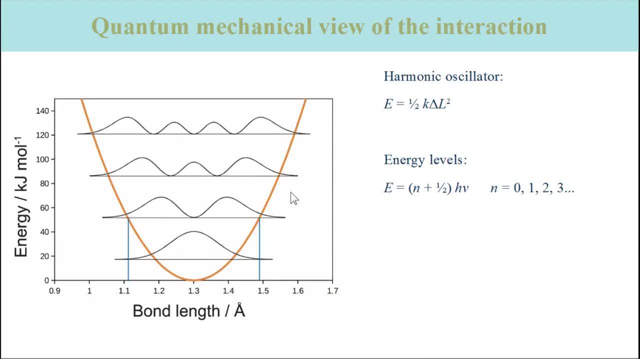 The total energy is represented by the horizontal lines in the figure for several vibrational states, Here, here, here here, Starting from the vibrational ground state, n equals zeros and up to n equals three. A classical oscillator moves between the two intersections of the horizontal line for the total energy, with the potential curve. 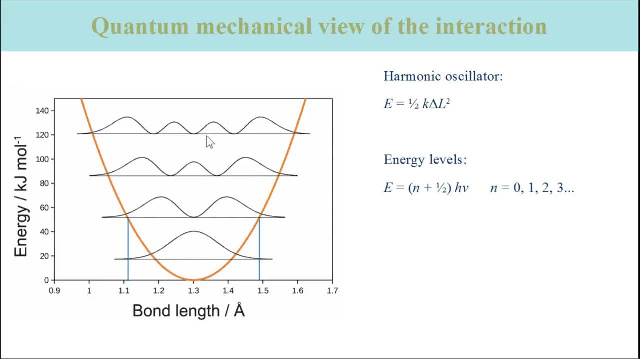 For example, a classical oscillator with a total energy that corresponds to the second energy level here would oscillate between a bond length of a bit more than 1.3.. and 1 ohmstroms to a bit less than 1.5 ohmstroms. 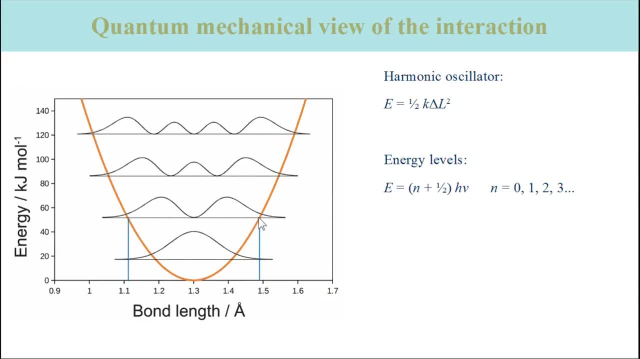 It cannot move beyond these limits because then it would move up the potential curve here and would need an energy that is larger than its total energy. This is different in the quantum world. For the quantum mechanical oscillator, the probability of finding the oscillating bond at a given bond length. 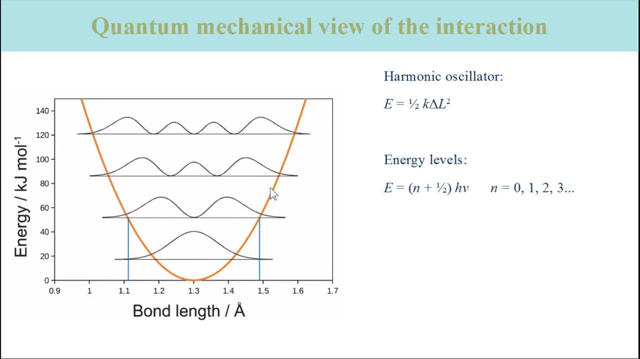 is shown by the curves on top of the horizontal lines. These ones, It can be seen that the quantum mechanical oscillator has a larger freedom to move than the classical oscillator, as the bond lengths can be found beyond the limits given by classical mechanics. Here and here.